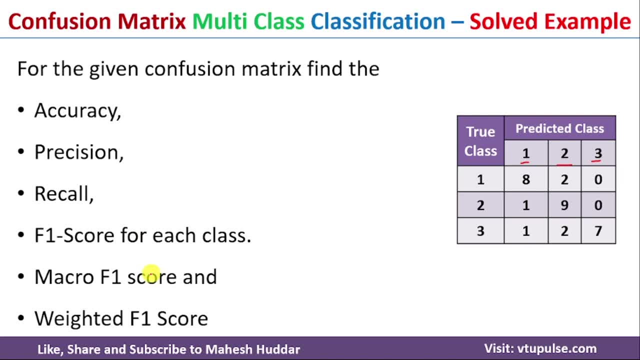 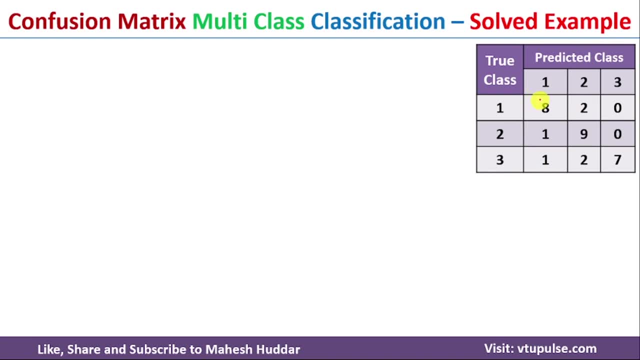 confusion matrix. we will try to calculate the different performance matrix here. Before we calculate the different performance matrix first, we need to convert this particular multi-class classification problems confusion matrix into binary classification problems confusion matrix. It looks something like this: Again, I have two classes on the vertical axis: predicted classes. 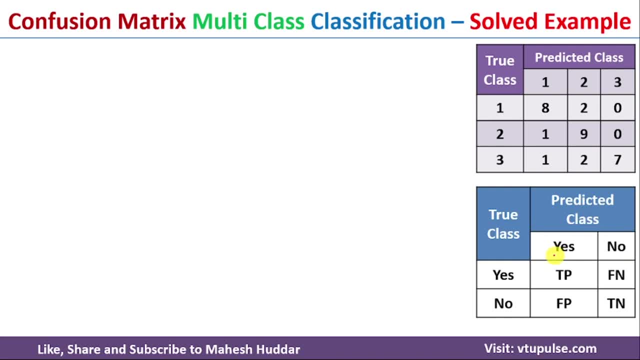 on the horizontal axis. This particular confusion matrix contains two classes. The first class is S and the second class is no, in this particular case. Now, if you look at this particular TP, TP is nothing but the number of S examples which are classified as S here. That is nothing but. 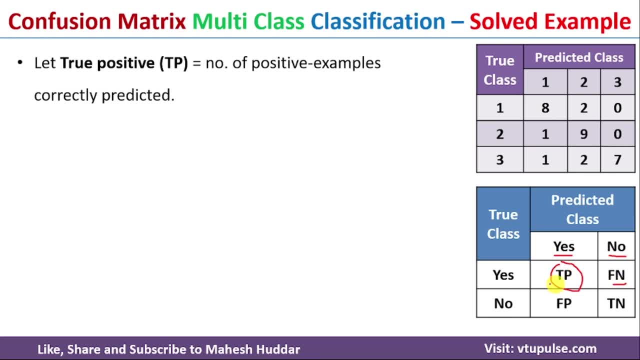 the true positive in this particular case. This FN is nothing but the number of S examples which were classified as no in this case. That is nothing but false negative in this case. Coming back to the third entry, that is, FP, That is nothing but the number of no examples which are classified as S, or you can say that wrongly. 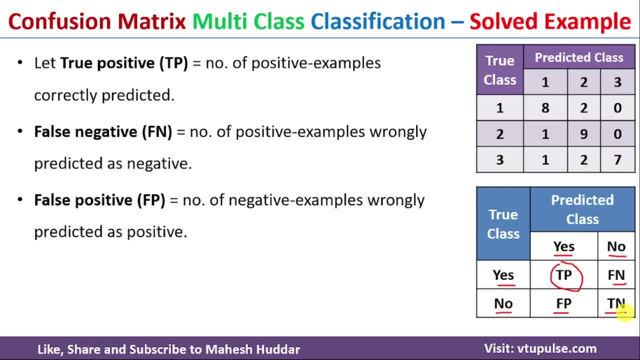 predicted over here. Coming back to the last one, that is, TN, TN is nothing but the number of no examples predicted as no over here or classified as no. That is nothing but the true negative in this particular case. Again, if you look at this particular thing, TP and TN are correctly classified or predicted. 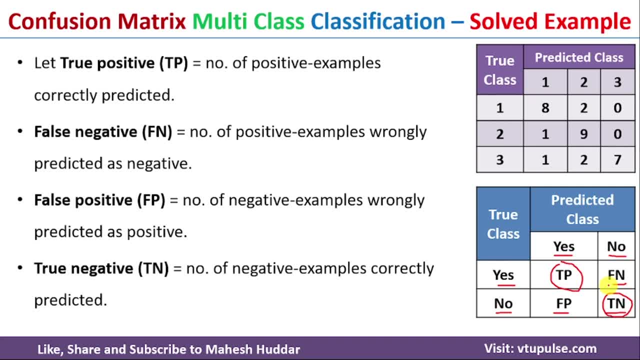 FP and FN are incorrectly predicted or classified in this case. First we will convert this multi-class classification confusion matrix into binary confusion matrix and then we will calculate the different performance matrix. Now the question comes in front of us is how to convert this multi-class classification confusion matrix into binary classification confusion matrix. 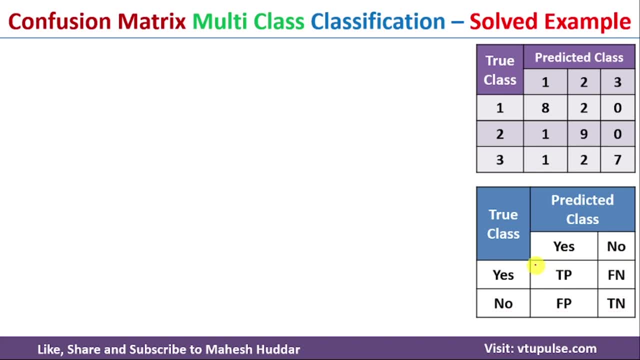 That can be done, Something like this. What we need to do here is first we will consider this class 1 as the S examples and remaining these two, that is, class 2 and 3, will be considered as no examples, and then we will get only two classes here, That is, class 1 as yes, class 2, 3 as no, in this case. 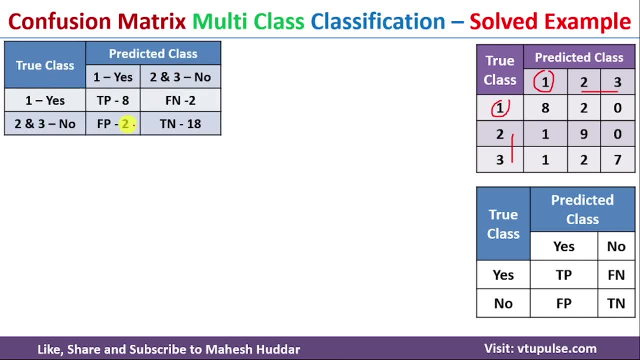 Now, once you get that particular thing, we will get the confusion matrix. something like this: 1 is yes here and 2, 3 as considered as no in this case. Now, if we look at this particular confusion matrix, the number of class 1 examples which were: 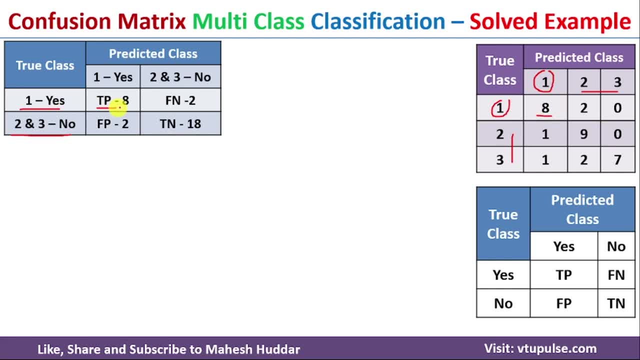 predicted as 1 in this case is 8 here. So that is what I have written as a true positive in this case, This 2 and 0, they are of type class 1, but they were classified as 2, 3 here. The meaning of: 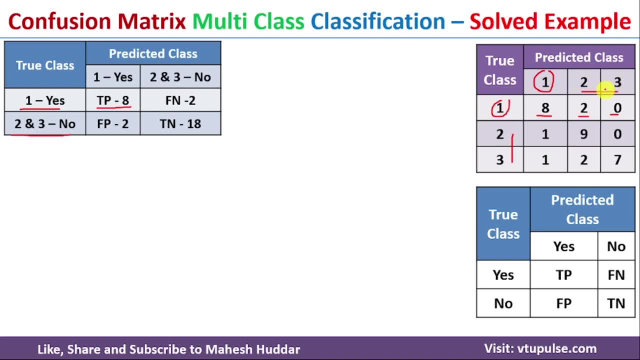 this one is: they are of type S examples, but they were classified as no. That is nothing but false negative. That is what I have written here. Coming back to these two examples, if you consider these two examples, these two are of type 2, 3.. That is nothing but false negative. That is what I have. 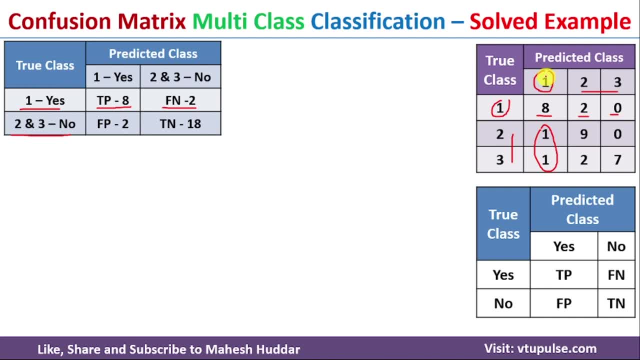 nothing but no examples. but they were classified as class 1.. That is nothing but yes. here. That is nothing but false positive. False positive will become 2. here And these four examples are of type. you can say that 2, 3 and they were classified as 2, 3. here The meaning is they were classified. 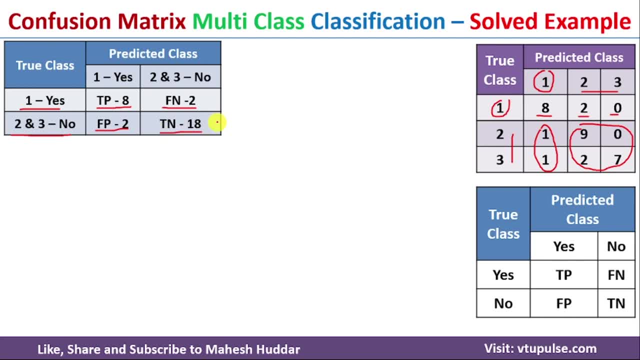 correctly, and it is true, negative here, which is equivalent to 18 in this case. Now I will consider 2 as the class S and then remaining 2, that is, 1 and 3 as the class no, And then I will try to. come up with a new class S, So I will consider 2 as the class S and then remaining 2, that is, 1 and 3- as the class no, And then I will try to come up with a new class S, So I will consider 2 as the class. 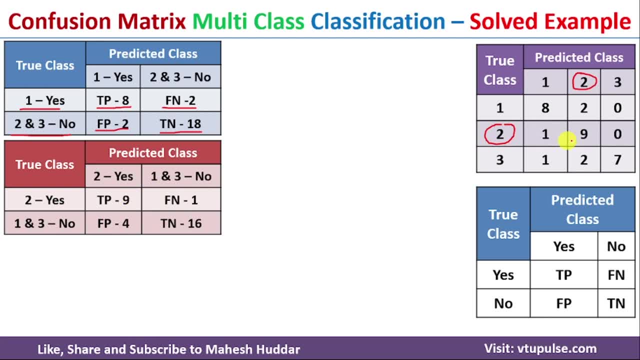 no, And then I will consider 2 as the class no And then I will consider 2 as the class no. Now, if you look at this particular matrix again, the number of two examples, or class 2 examples, which were predicted as 2, are 9 here. So that is what you can notice here And I have written it. 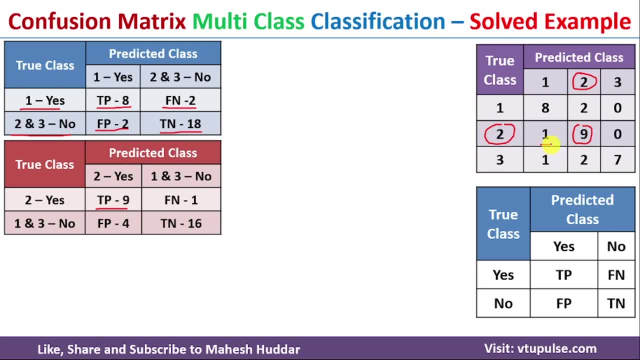 here. that is true, positive in this case. If you look at these two numbers, that is, 1 and 0, they are of type class 2, but they were classified or predicted as 1, 3. here The meaning is it is a. 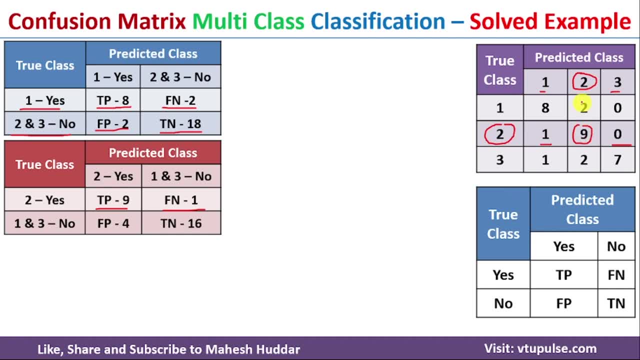 false, negative in this case. And if you look at these two numbers, that is, this 2 and this 2, they are of type 1 and 3, that is nothing but no examples, but they were predicted as 2 here. 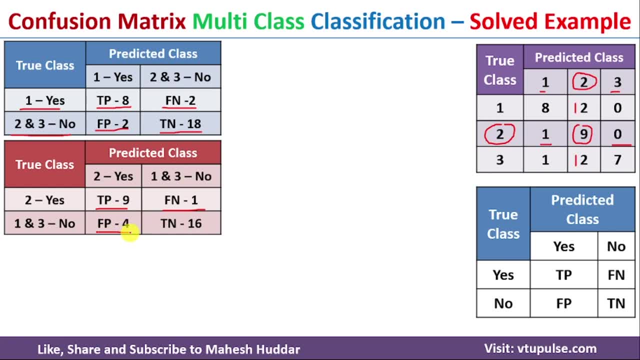 that is nothing but yes in this case. So it is nothing but false positive here. And these four- this is 8,, 0,, 1 and 7, they are of type 1, 3 and they were classified as 1, 3.. The meaning is no. 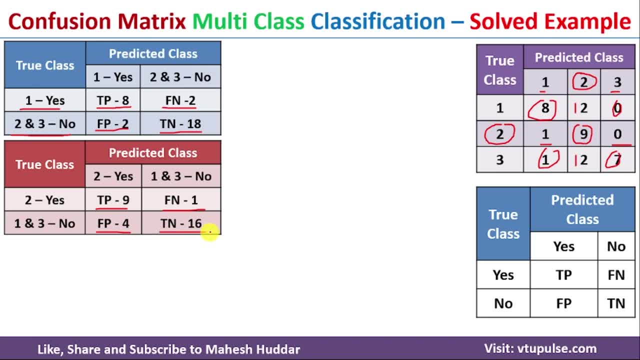 examples were predicted as no. that is nothing but true. negative, which is equivalent to 16 here. Similarly, we need to create one more confusion matrix For the third one, where 3 will be considered as yes and 1, 2 will be considered as no. here, 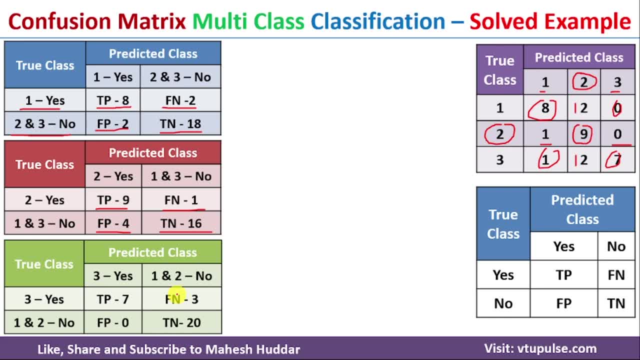 And it looks something like this: Once you form this confusion, matrix for binary classification. now we will try to find the values for each of those particular performance matrix. The first one in this case is accuracy. Accuracy for class 1 is equivalent to tp plus tn. 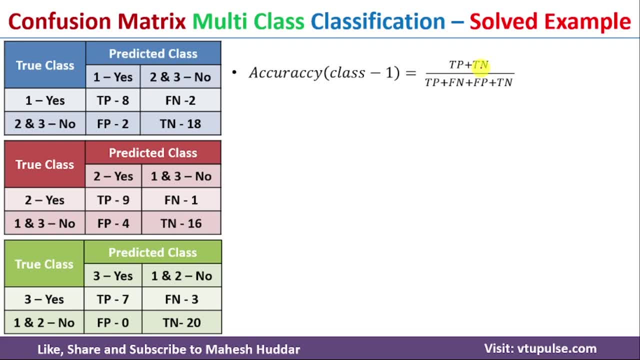 that is nothing but true positive plus true negative. that is the correct classification. divided by all, Then tp plus tn plus true negative. Once you put the values from the particular confusion matrix into this equation, you will get 0.87 as the accuracy for class 1 here. 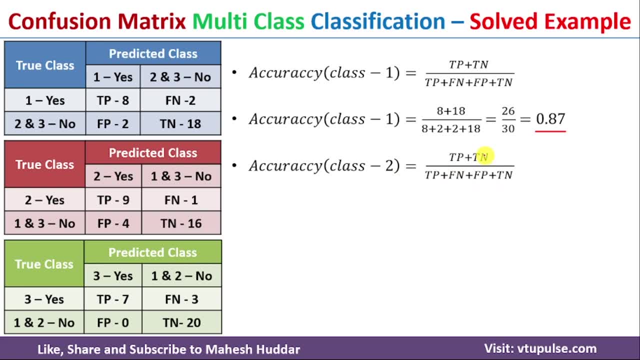 Similarly, we will calculate the accuracy for class 2.. Again, we need to use the same equation, but the values. we need to use it from this particular confusion matrix. here we will get 0.83 as the accuracy for second class. similarly, for the third class, we need to use the values from: 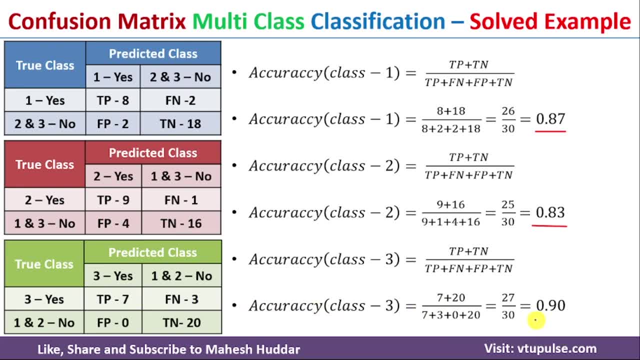 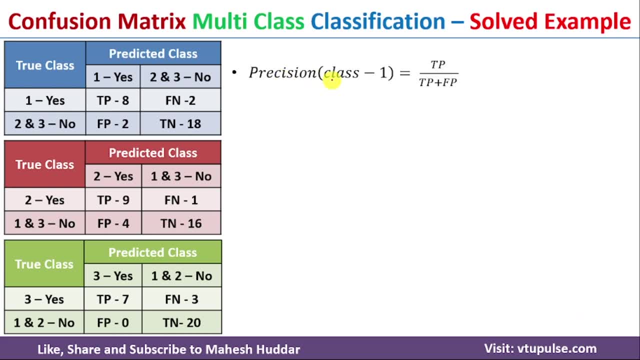 this particular matrix, we will get 0.90 as the accuracy in this case. now we will try to calculate the remaining performance matrix. precision of class 1 is equivalent to tp divided by tp plus fp, so i will put the values here again. i will get the value as 0.8 for a class 1 precision. similarly, we 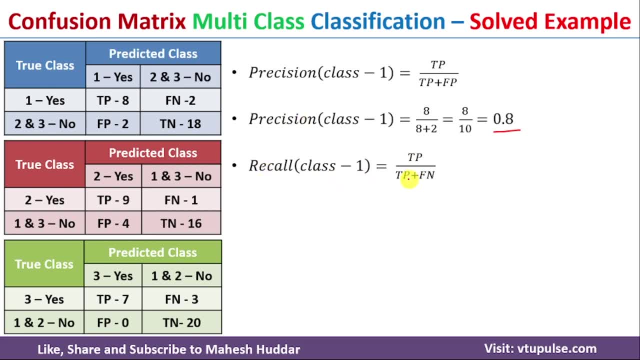 will calculate the recall for class 1, which is equivalent to tp divided by tp plus fn, which is equivalent to 0.8. once you calculate precision and recall for class 1, we can calculate the f1 score for class 1, which is equivalent to 2 times precision multiplied by recall, divided by. 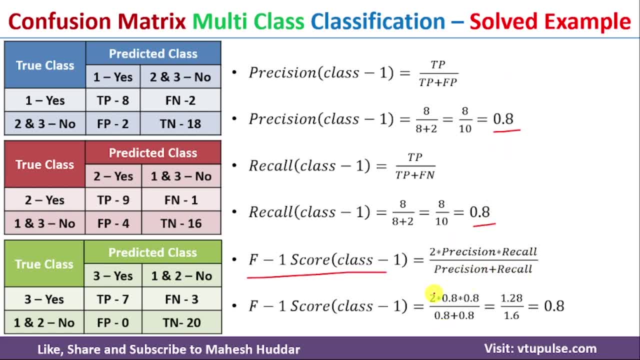 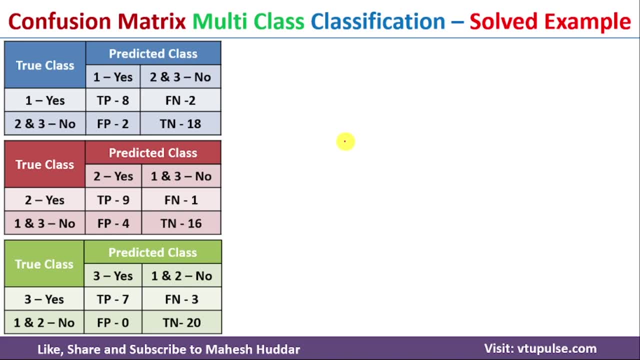 precision plus recall. we have these values. we will put those values and then we will get 0.8 as the f1 score for the class 1 over here. similarly, i will calculate the precision for class 2. i will put the value from this one into this equation. i will get. the precision for class 2 is equivalent to 0.69. 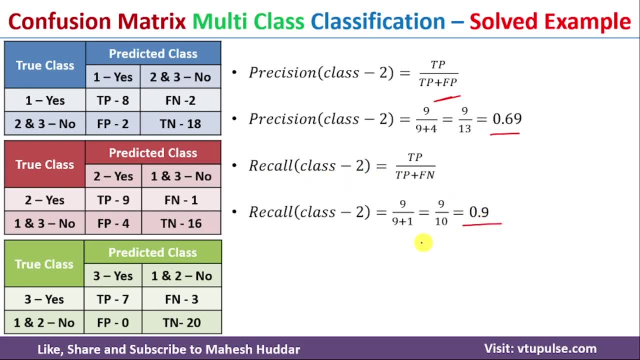 similarly recall for class 2 is equivalent to point 9 and the f1 score for class 2 is equivalent to 0.78. here, once you're done with the class 2, i will go with class 3. again the same equation. only thing is we need to put the values from.